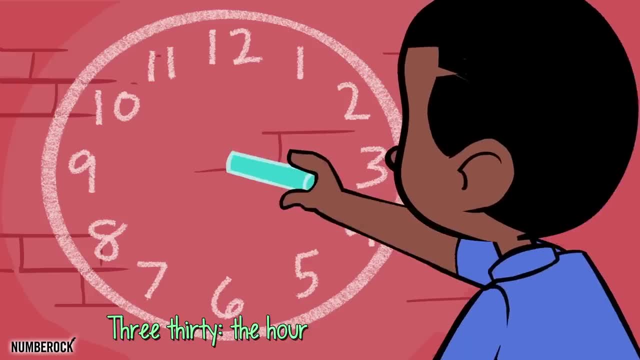 whether breakfast or sup. If the hour hand's on a number, We know it's o'clock, whether breakfast or sup. If the hour hand's on a number, We know it's o'clock 3.30,. the hour hand is half past three. The minute hand's at six, halfway round which. 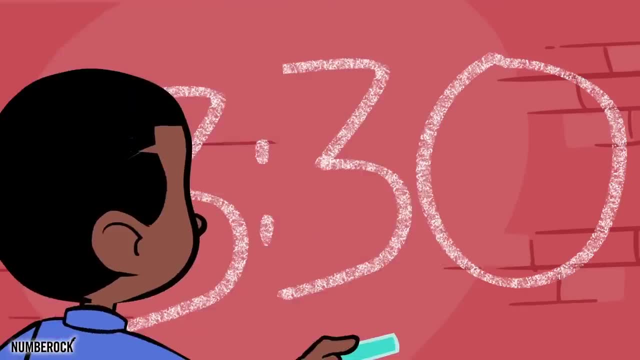 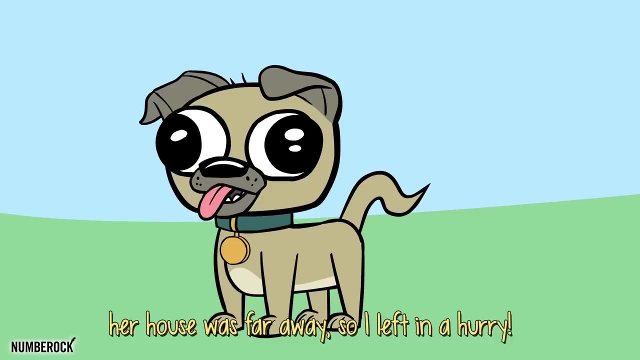 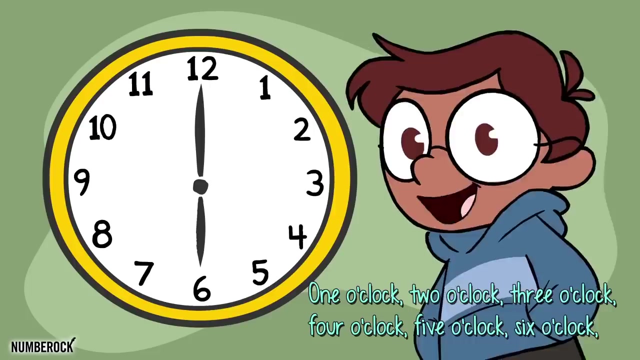 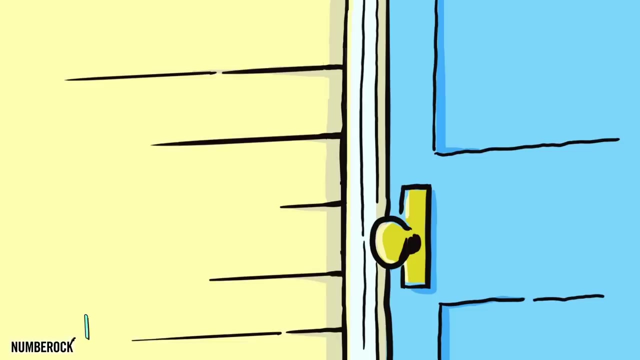 is 30. I remembered I had to meet my friend Lexie. Her house was far away so I left in a hurry, A hurry, A hurry. 10 o'clock, 11 o'clock, 12 o'clock. I got to Lexi's door and then rapped. 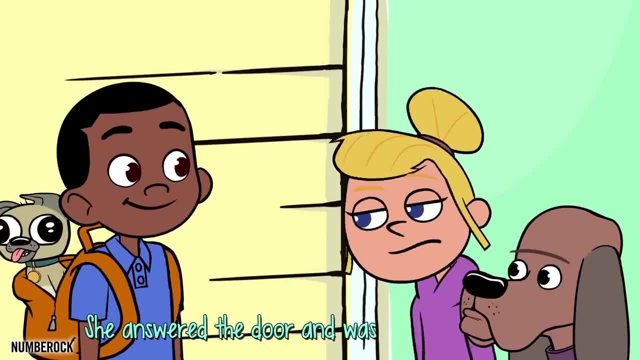 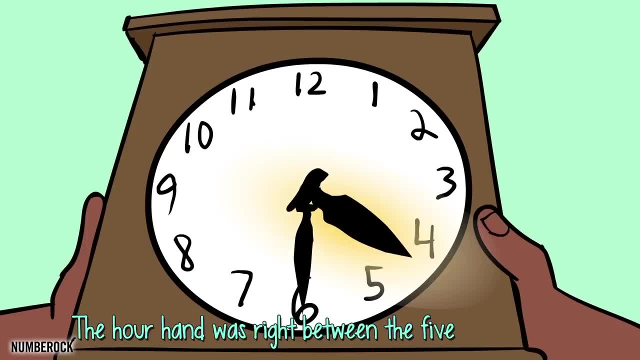 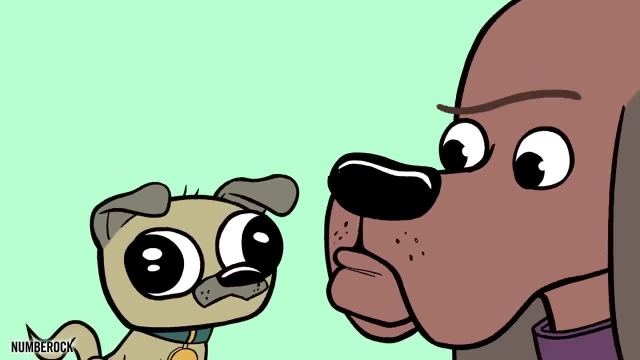 Knock, knock. She entered the door And was pointing to the clock, Tick-tock, tick-tock, tick-tock. The hour hand was right between The five and the four. The minute hand was at six, Pointed down toward the floor. Oh, yeah, yeah. 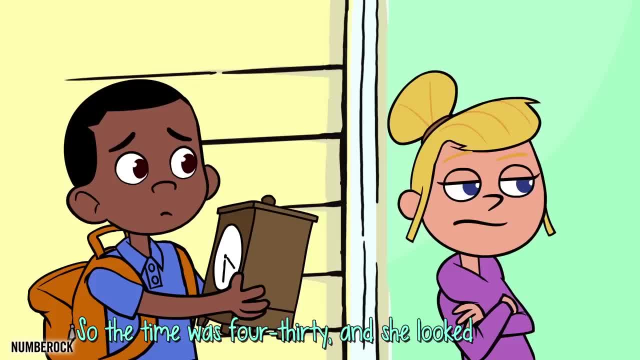 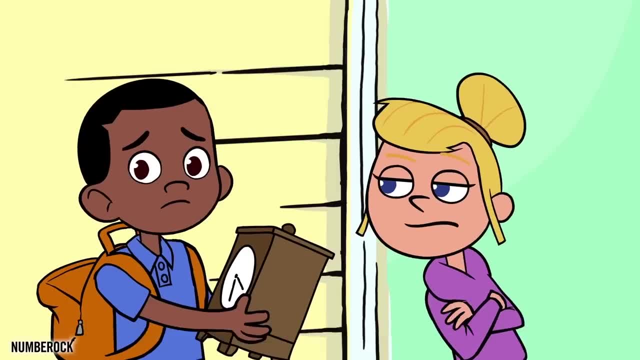 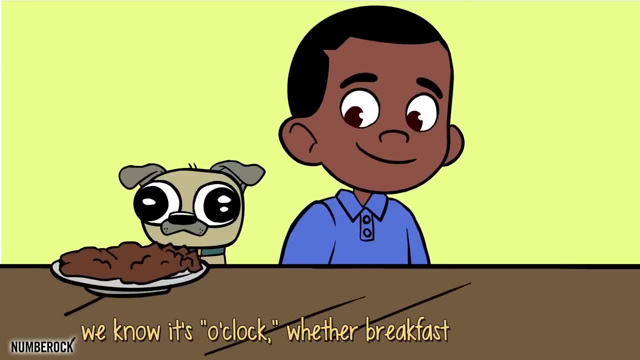 So the time was 4.30 And she looked annoyed. You said you'd be coming no later than four. Oh boy, When the hour hand's on a number And the minute hand's up, We know it's o'clock. Where the breakfast? or a sub? Oh, yeah, yeah. 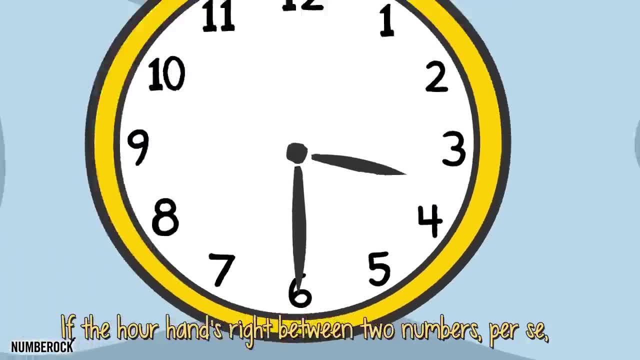 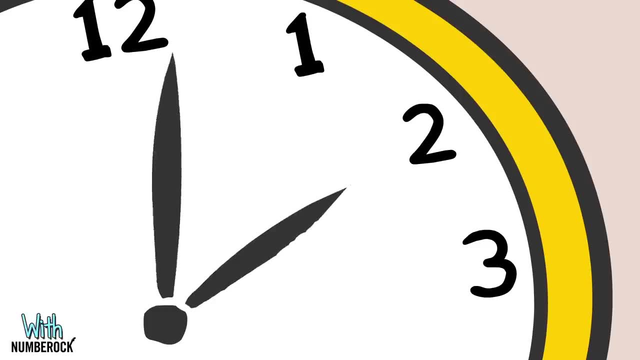 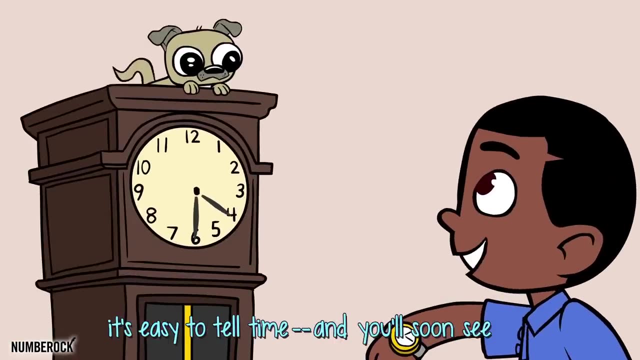 If the hour hand's right between Two numbers per se, It's half past the hour, All 3.30 that day. With the long minute hand That represents The hour hand. As the minutes go by, It's easy to tell time And you'll soon see why. 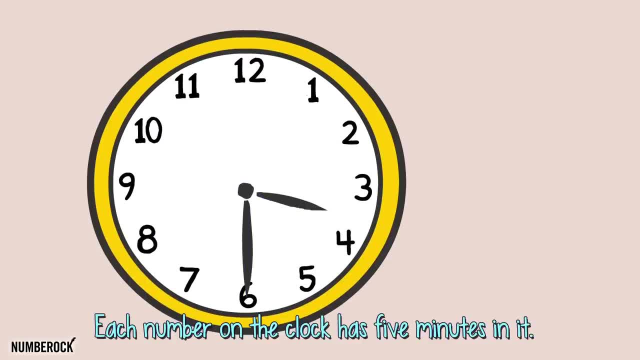 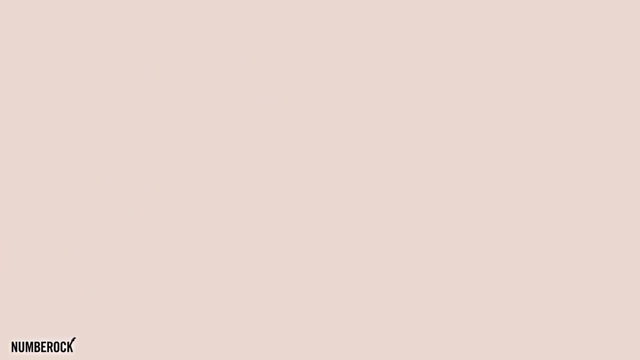 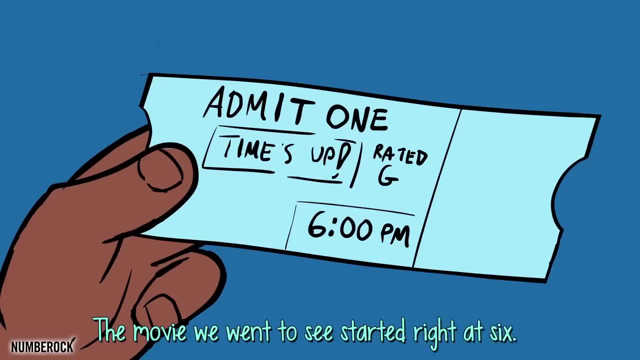 Each number on the clock Has five minutes in it. If you skip, count by five, You'll tell the time. Lickety split. We went to the movies And they bought us two tickets. The movie we went to see Started right at six. The hour hand Was at six. 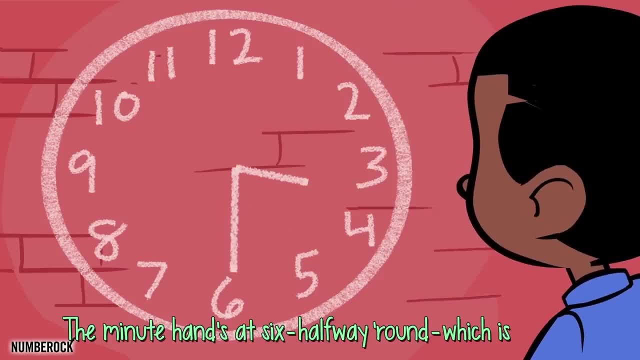 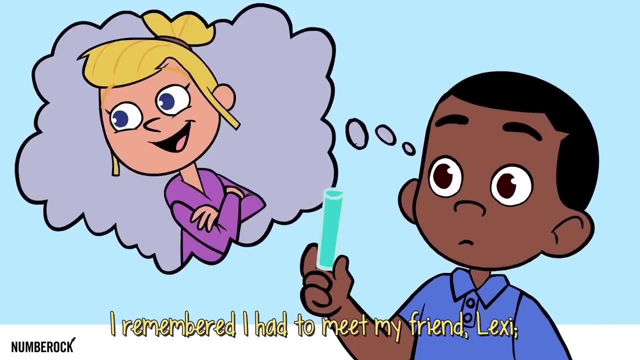 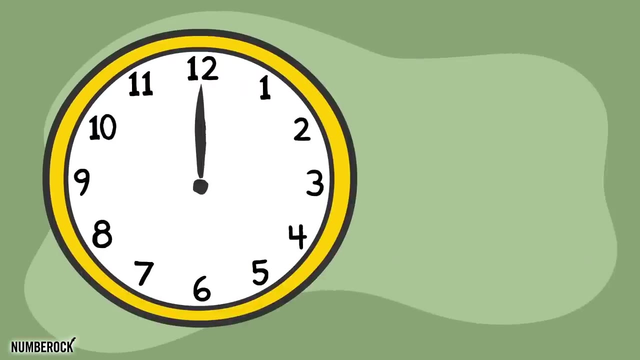 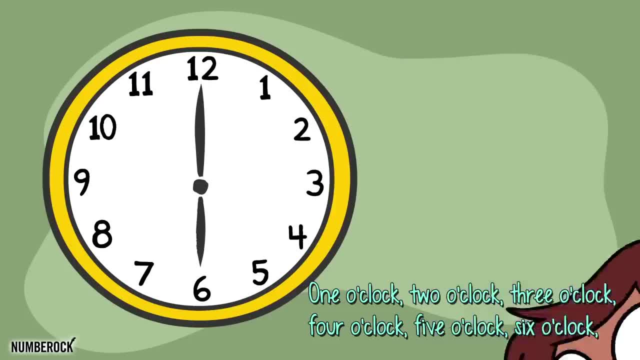 1 o'clock, 2 o'clock, 3 o'clock, 4 o'clock, 5 o'clock, 6 o'clock, 7 o'clock, 8 o'clock, 9 o'clock, 10 o'clock, 11 o'clock, 12 o'clock. 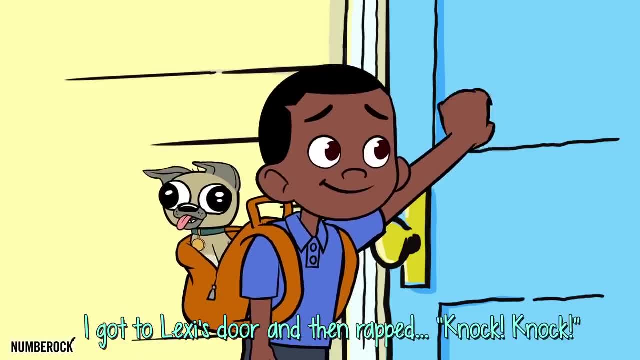 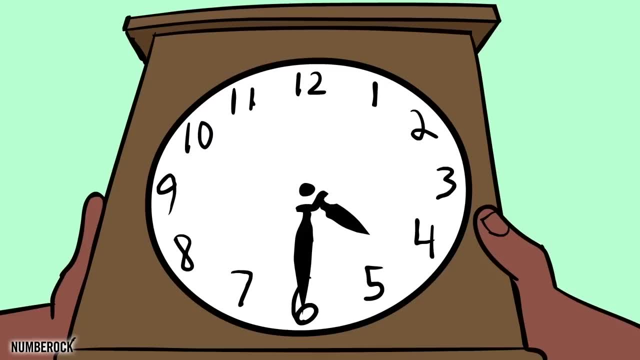 I got to Lexi's door and then rapped, Knock, knock. she entered the door And was pointing to the clock: Tick tock, tick tock, tick tock. The hour hand was right between The five and the four. The minute hand was at six. 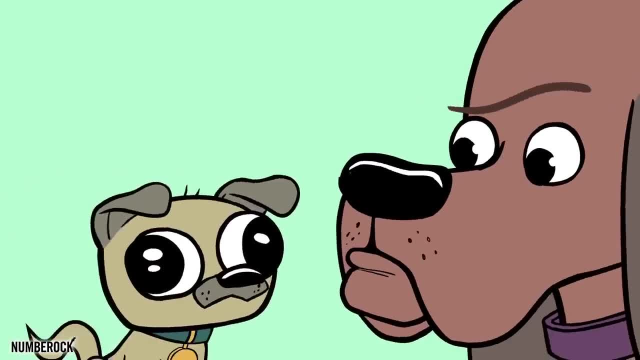 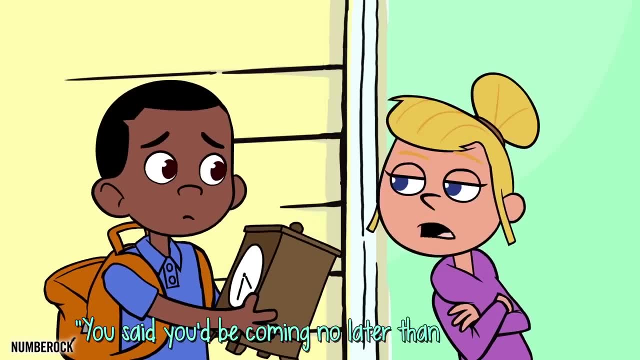 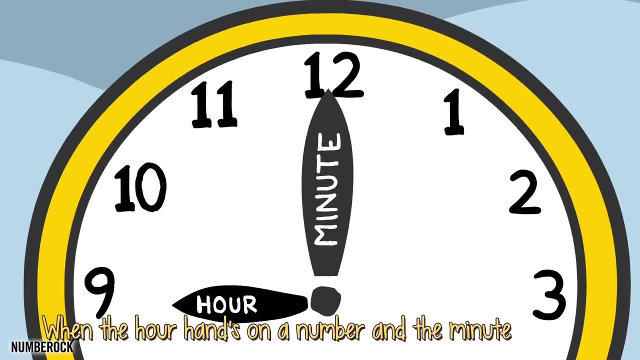 Pointed down toward the floor. Oh yeah, yeah. So the time was 4.30 And she looked annoyed. You said you'd be coming no later than four. Oh boy, When the hour hand's on a number And the minute hand's up, We know it's o'clock. 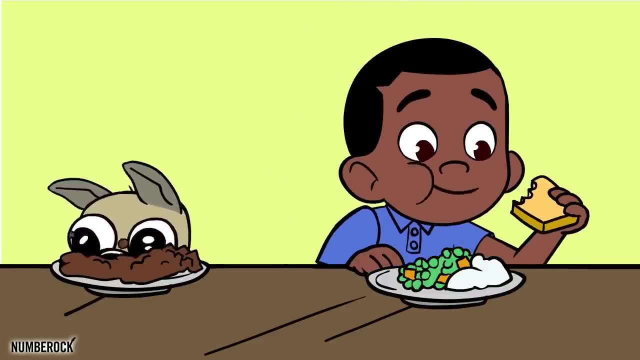 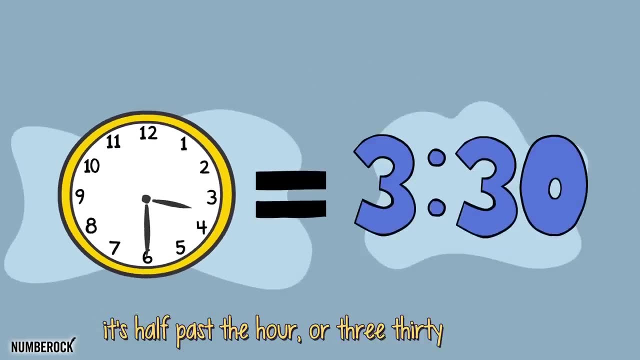 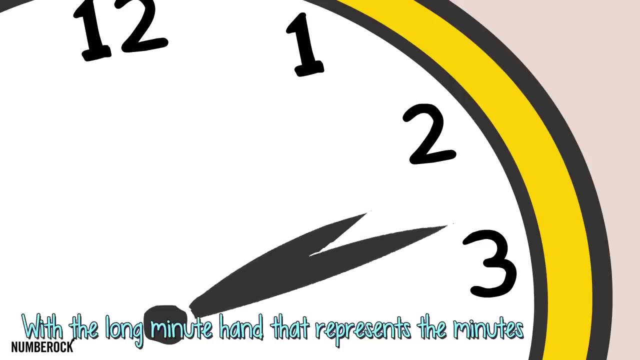 Whether breakfast or a sub. If the hour hand's right between two numbers per se, It's half past an hour, All 3.30 that day. With the long minute hand That represents the minutes gone by, It's easy to tell time, And you'll soon see why. 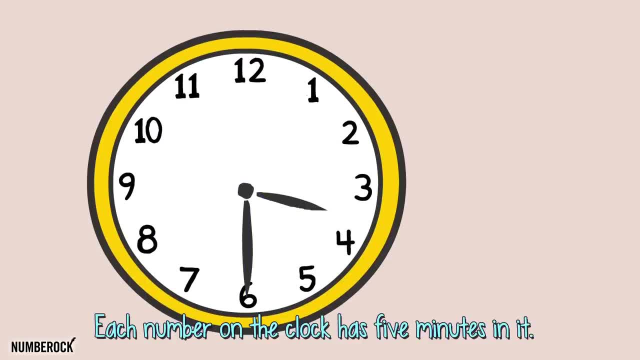 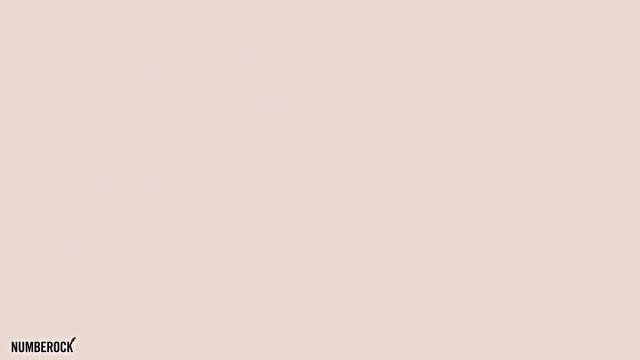 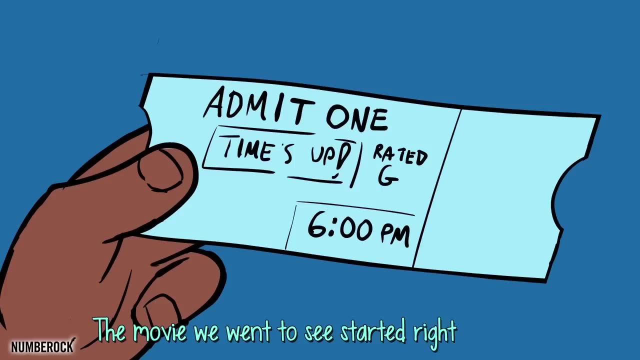 Each number on the clock Has five minutes in it. If you skip, count by five, You'll tell the time. Lickety split. We went to the movies And they bought us two tickets. The movie we went to see Started right at six. The hour hand was at six. 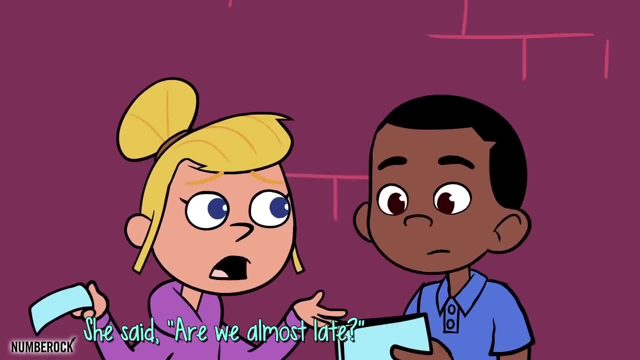 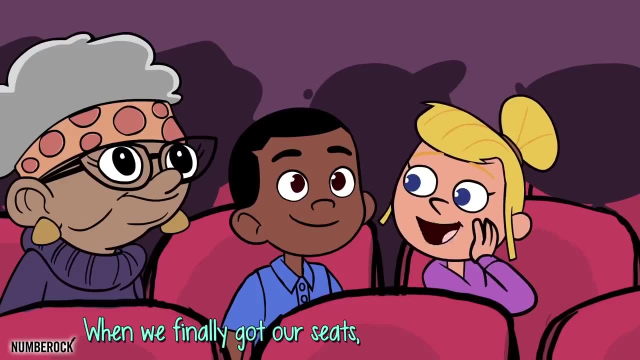 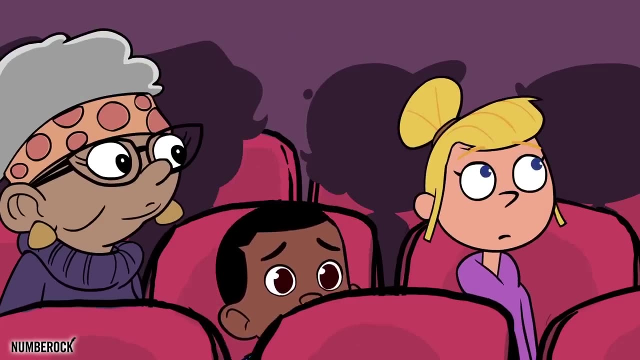 The minute hand pointed up, She said: Are we almost late? And I was like, Yup, Oh yeah. When we finally got a seat, She told me I was cute But I'd eaten beans for lunch And let out a loud toot. Oh no, no, no, no. 12.30.